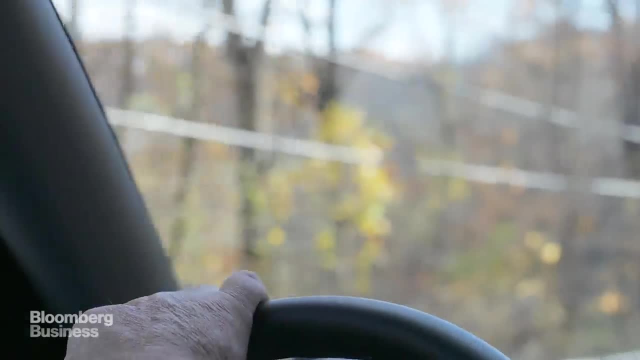 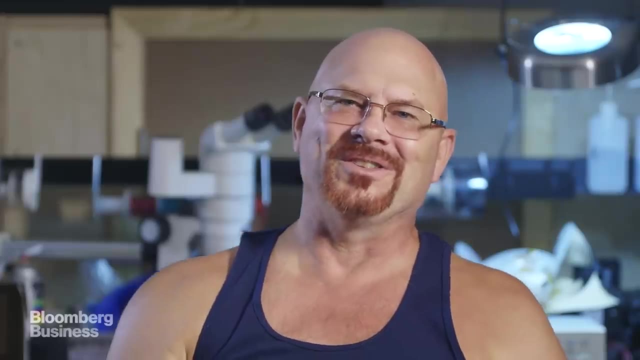 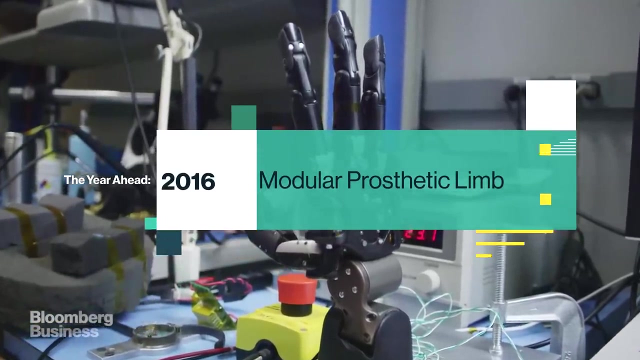 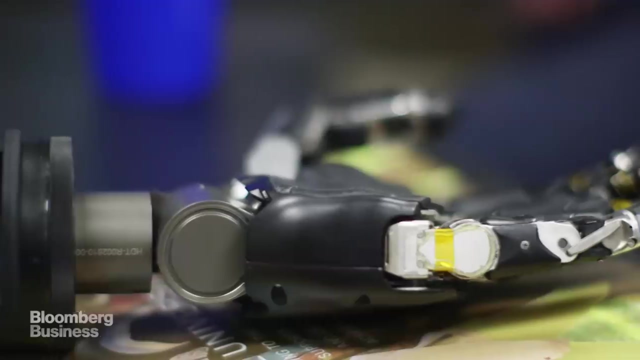 newest thing in prosthetics: It's an implant. They said, well, do us a favor, Just don't put your arm out the window until you get your prosthetic on there. So we got more things to do than keep pulling you over. I used to be a salesman. 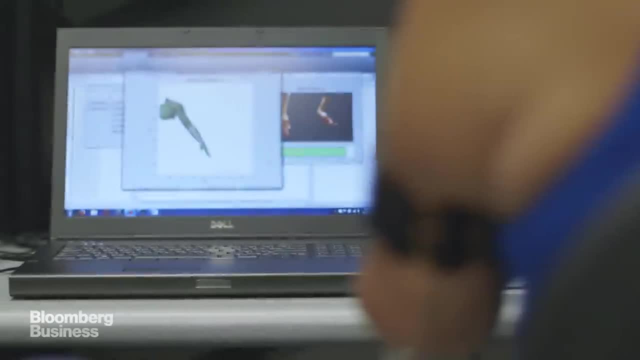 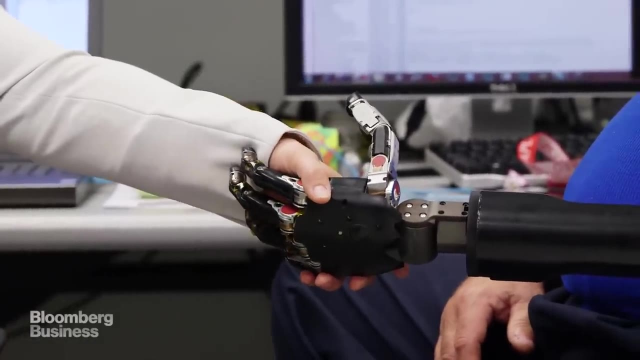 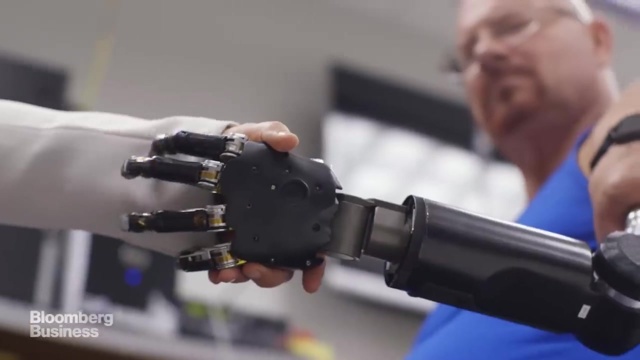 and in. In 2005,, I was diagnosed with having cancer in my left forearm. It was so aggressive it just wouldn't even slow down. So in 2008, I had an amputated arm just above the elbow. I got a second chance of life. 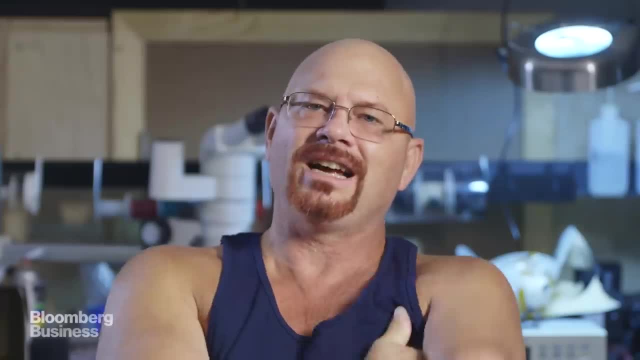 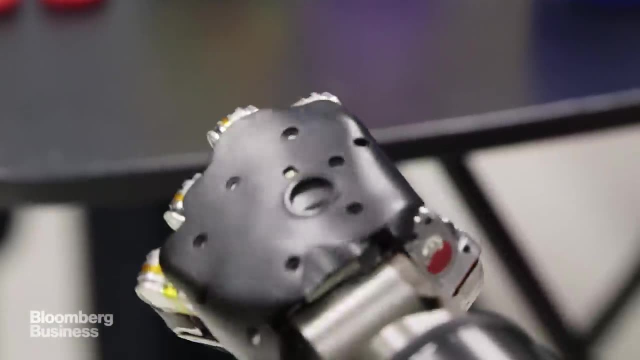 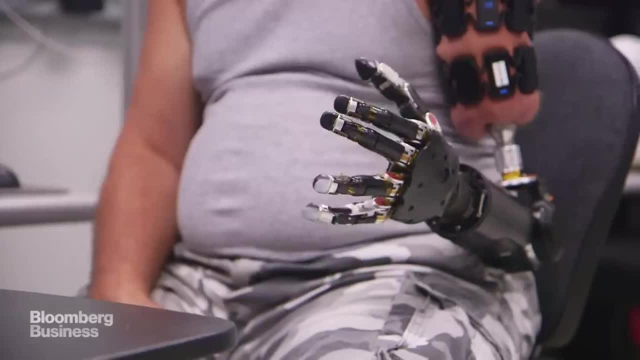 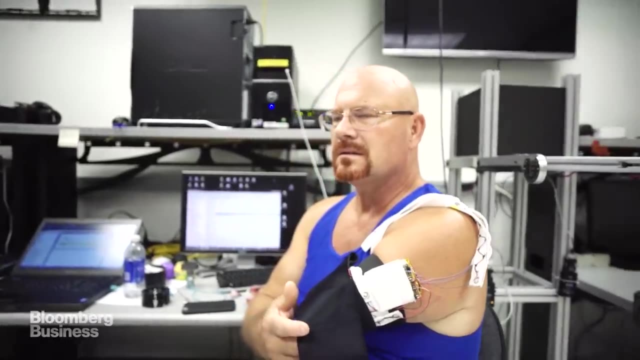 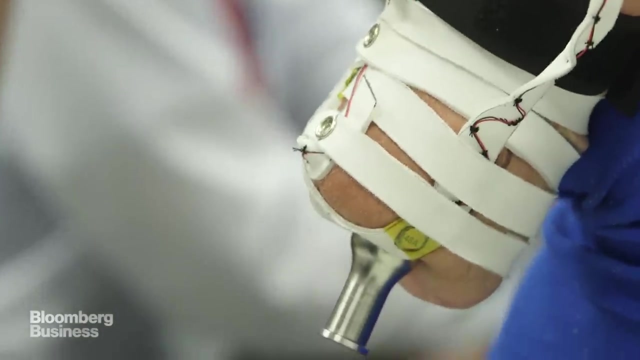 Hand open. What he's testing here, here being the Johns Hopkins Applied Physics Laboratory, is a glimpse into the future of how humans and machines interact. It's a mind-controlled arm that attaches directly to his skeleton, And it's the result of a decade of work and $120 million of military funding. 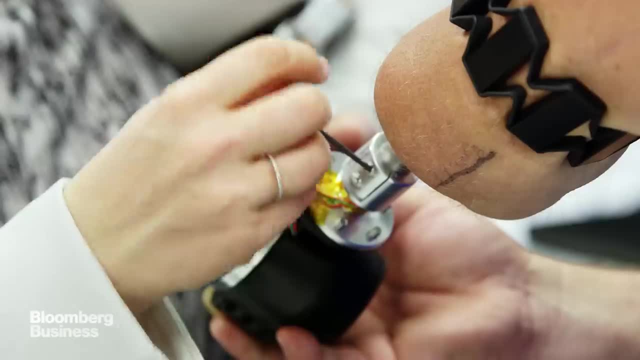 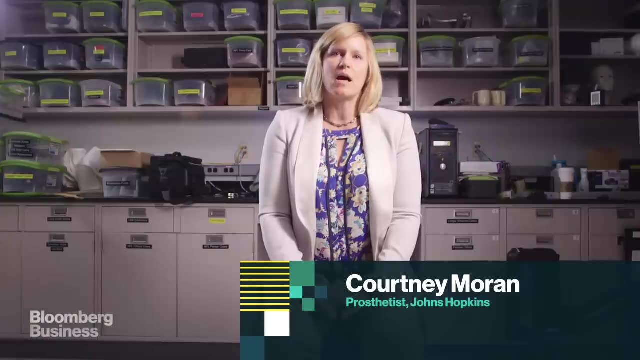 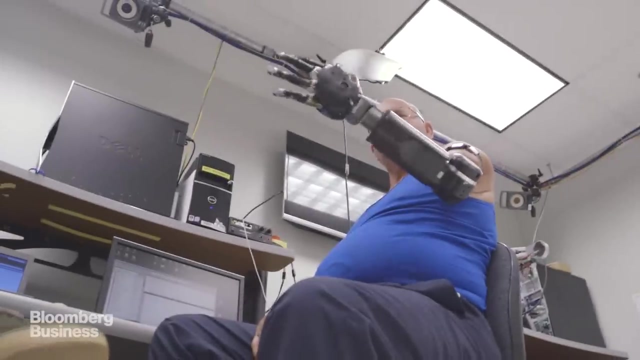 So this is the first time that we're attaching a prosthetic device to an implant that protrudes out of his skin and allows the prosthesis to actually be physically attached to his skeleton. Okay, elbow extend, Elbow bend. I had a problem with all the arms that I was working with. 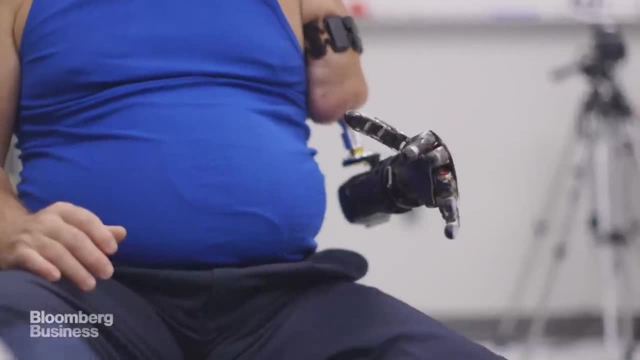 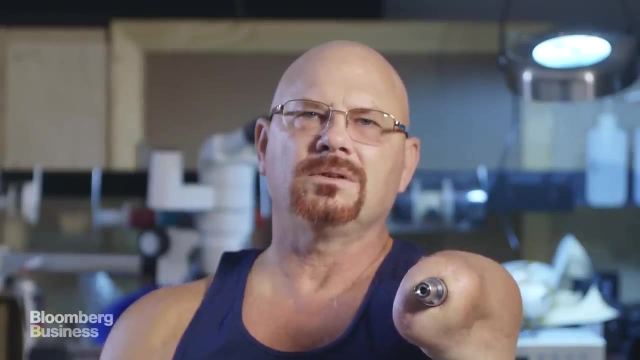 I was having skin breakdown on my stump. With osteoagration, you don't have to worry about the suction on the stump, It connects directly. It connects directly to the implant, and so, therefore, you can continue wearing it no matter what. 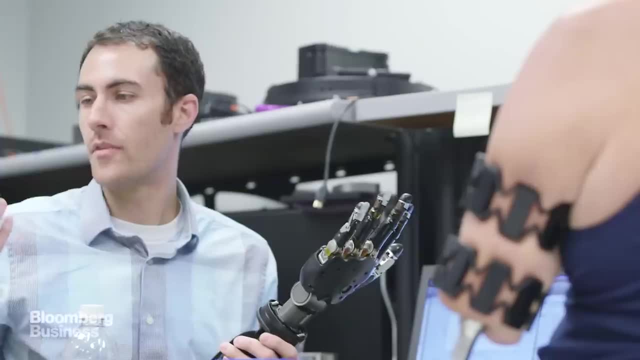 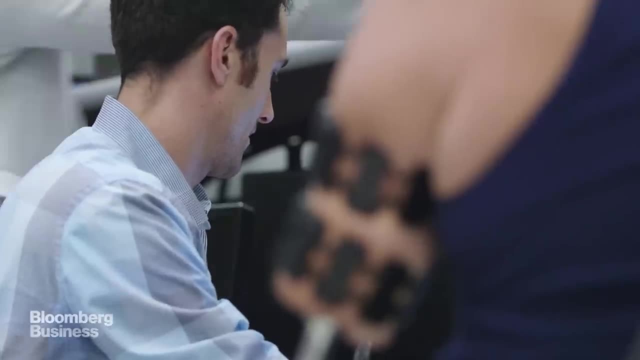 Johnny's implant allows for more strength and mobility, but maybe more impressive is he can control the arm with his thoughts. For this he had to undergo another surgery to rearrange the nerves from his missing arm. All right, so we'll start with no movement. 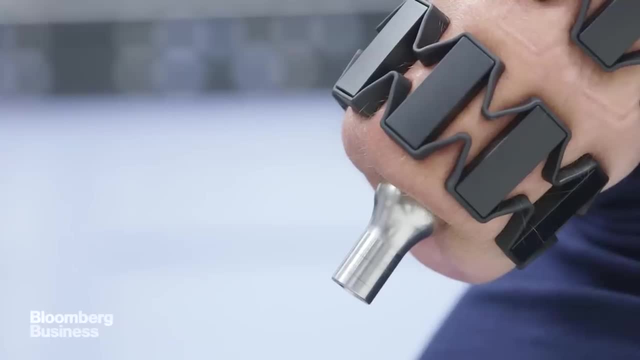 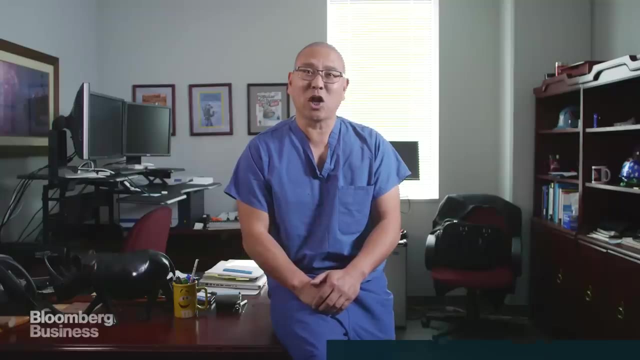 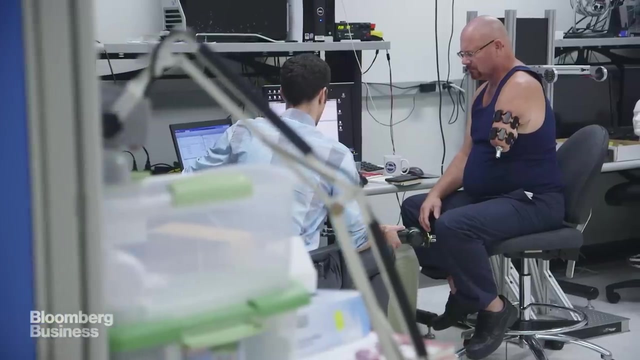 Ready? That's, pronate, Supinate, Go. We are actually witnessing something that has never been seen before, Done before. Is Johnny really controlling that limb simply by thinking about it with normal intuitive thought? We are using wireless myobands to transmit that muscle activity. 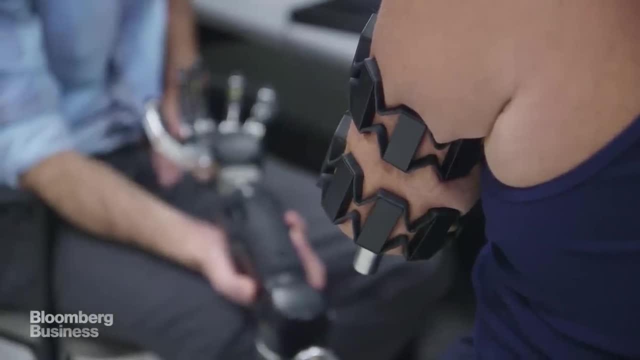 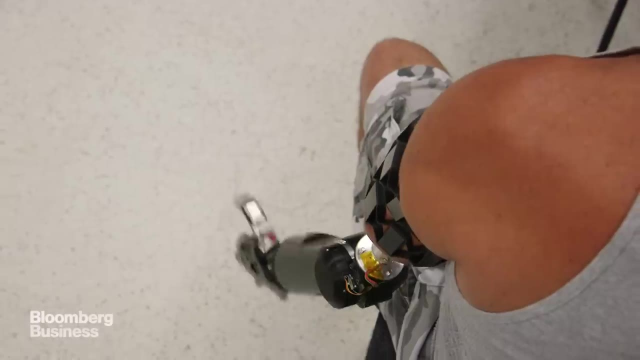 So now, when he thinks of moving his missing limb, it now contracts those newly re-innovated muscles: Elbow flexion: Ready And go. Hand open And go. Wrist rotate in And go Ready And go. 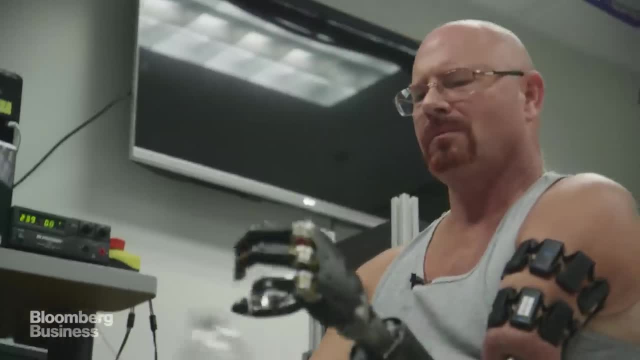 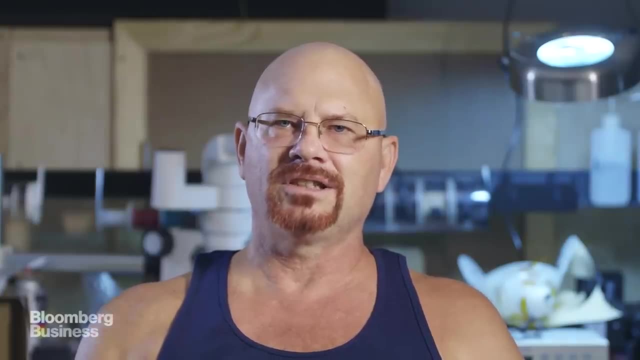 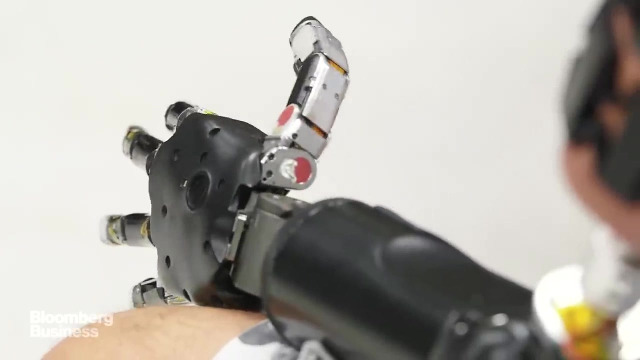 And go And go. It's hard. I've done hundreds of thousands of hours of mental exercises just trying to do the different grips, bends, rotations, points, pinch. So anyone that you know, right after the surgery they think they can step right back into it and, you know, just start working it. 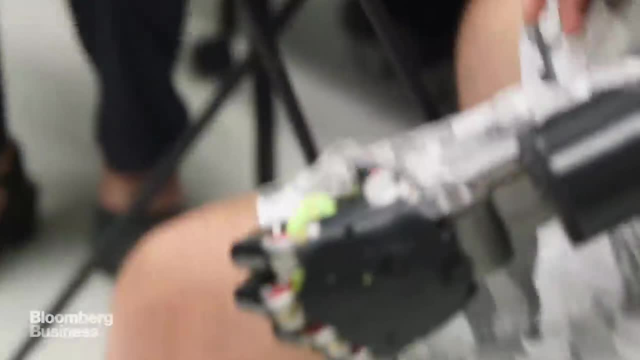 I mean, you know you're in for a rude awakening. It takes a lot of time. You want to hand that to me? I'm not. You're going to be fine. You're going to be fine. You're going to be fine. 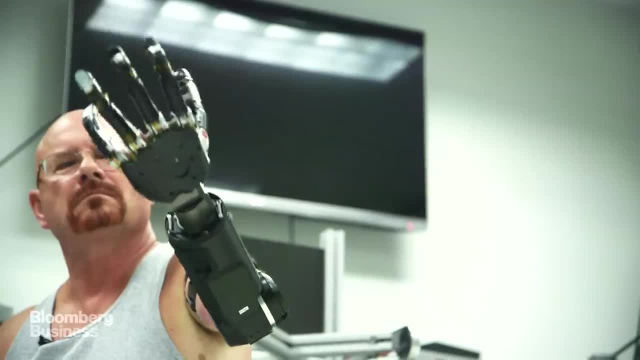 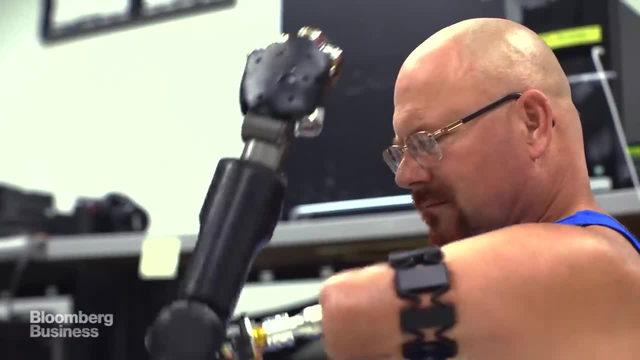 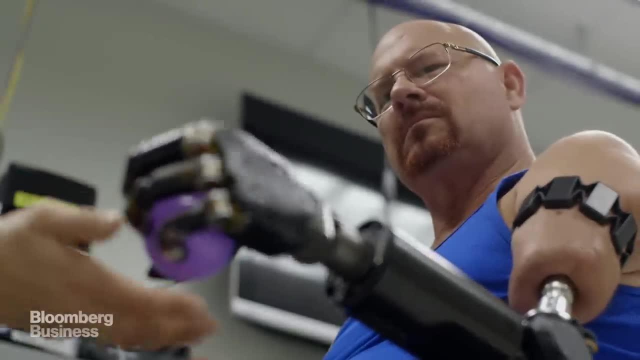 Soon, he'll be able to feel how hard or soft something is, to understand its texture and even its temperature. As he moves forward, Johnny represents a future where robotics goes from being a tool we use to actually becoming a part of us. I want the ultimate arm. 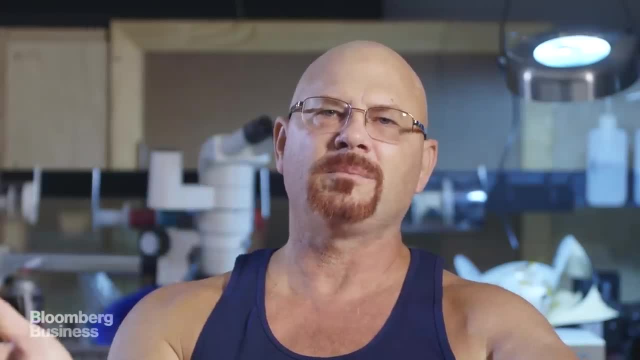 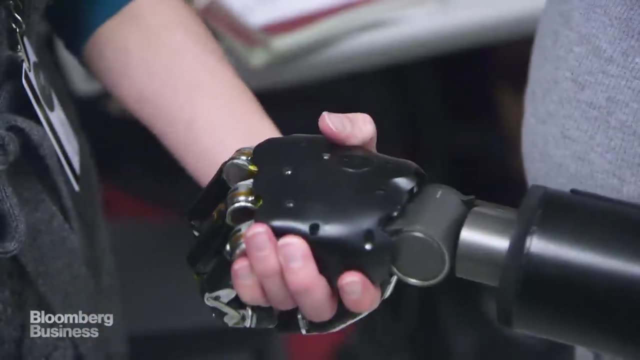 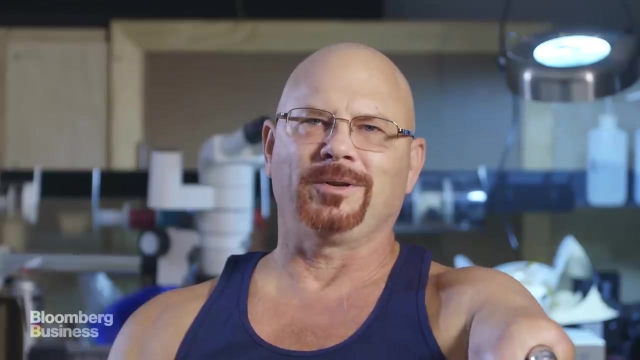 I want it to be as near natural as a human arm as possible. You trust me? Yes, Hand, shake me. How you doing Good Good to meet you. I'm like the Model T of cars, or I'm the Wright Brothers of airplanes. 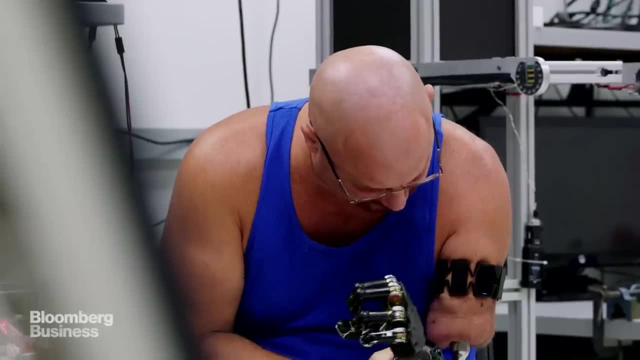 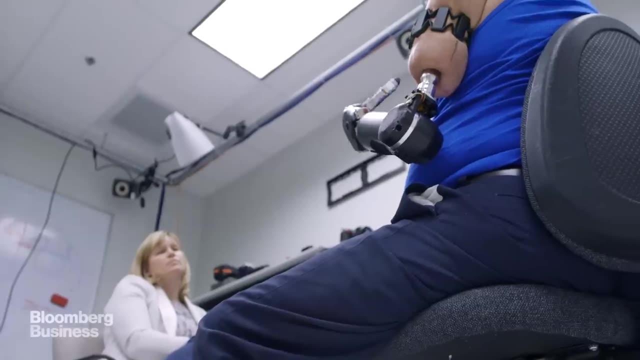 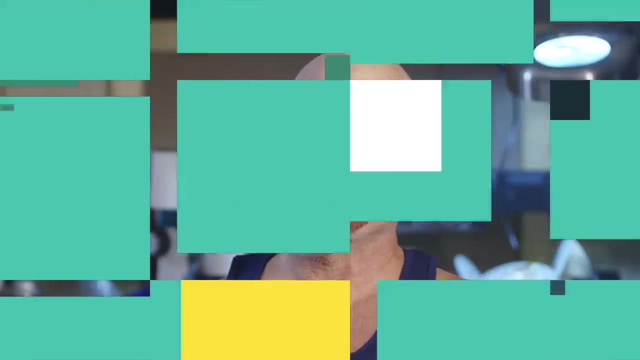 You know I'm the beginning And as we progress then you're going to see us can finally move up to the Maseratis or these supersonic jets. So we're going to say back to the future has begun.